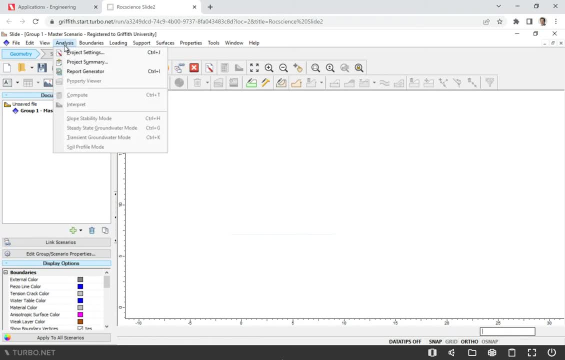 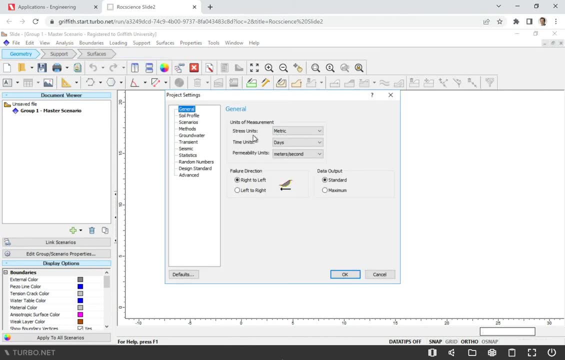 next step, which will be analysis, And first of all we'll start with project settings. So project settings first, we'll make sure that we have metric units, And then failure direction. This is very important. Sometimes people make mistakes. Well, they don't really make mistakes. Some software. 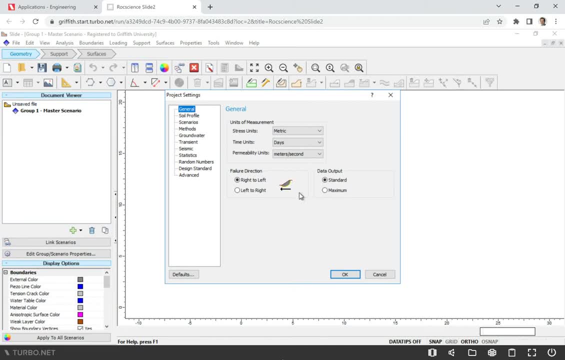 doesn't work, It's because for this setup, you will see that you will need to draw the top of the slope on the right-hand side And the slide will be in this direction, from the right to the left, left. so if, for some reason, you drew a slope which is top on the left and the 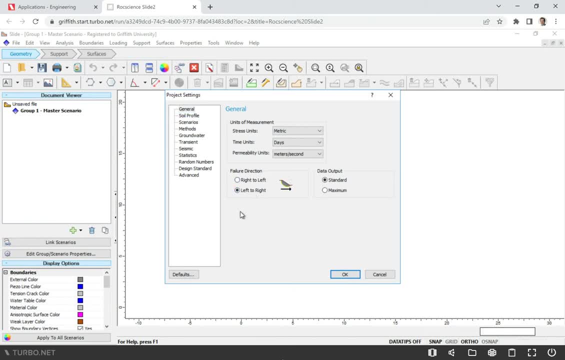 slide will be from left to the right. you have to change the failure direction. so just remember this one, because sometimes students ask me how come it doesn't work? well, it doesn't work because the failure direction is wrong. so this is very easier to fix. even if you make mistake at first, you just come here and change. 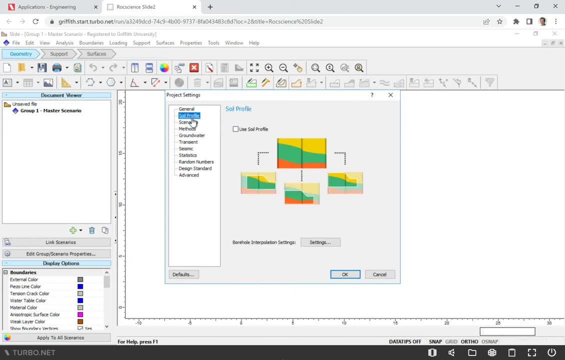 okay, next one, soil profile. well, probably you don't need this one. scenarios: this is, I think, improvement compared to the previous version. you have multiple scenarios. I tried to use it some. I think the good thing is you can maybe play with different cases, like you can change ground water table. 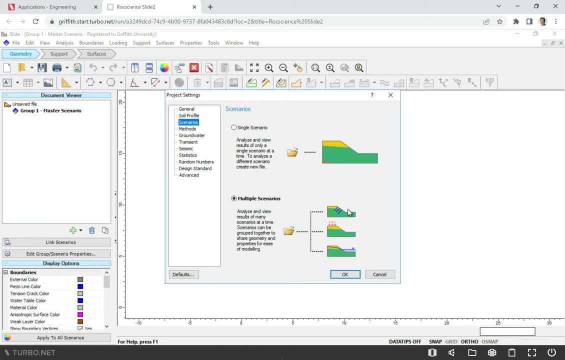 you can change ground water table and you can change soil profile and you can change soil profile and you can change soil profile and you can change soil. unfortunately, you cannot change the property, so the properties will be the same for all these scenarios. so I'm not sure if it's that useful. so well we're. 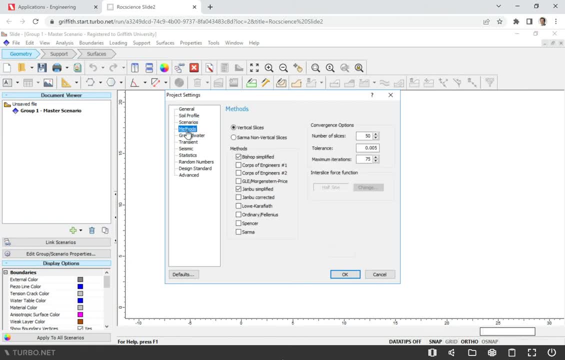 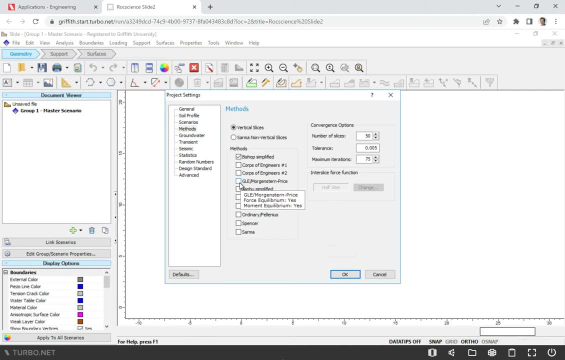 can you know the theory behind this first method? you know you can change more into slice back this way and you can change pierws World number of slices. you know there will be half sign and when you have a number of for limit, equilibrium method analysis software will divide, slope into slices. 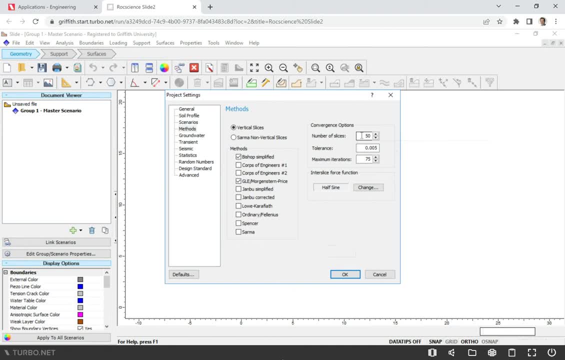 in this case preset as 50, so it will be 50 slices. I think 50 is too many. I'll just change to 25. but it's up you: 25, 30, 50. I don't think it will change the analysis very much. I don't think it actually will affect it. okay, so that's. 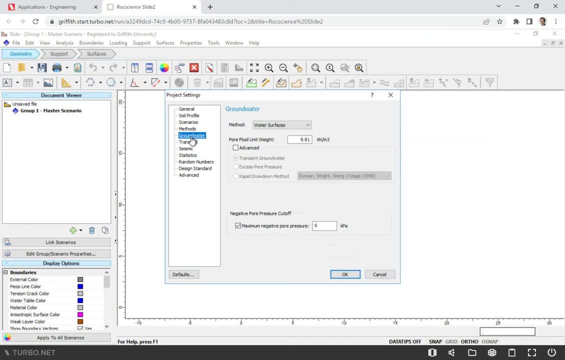 about it. ground water don't really need to change anything here. we're gonna go with just ground water table seismic: we don't any data on seismic coefficient, so we're not going to use this option as well, so I'm gonna click OK. next step is we're going to draw a slope, so we need to know slope geometry. you need to know. 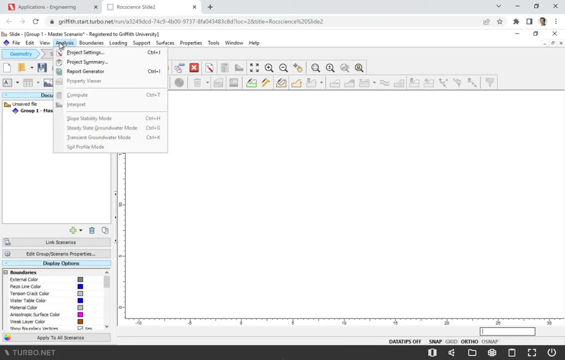 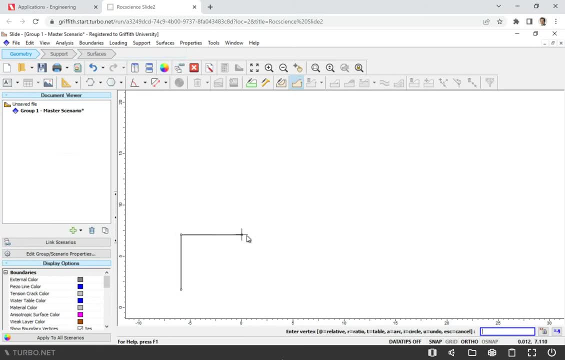 a slope, so remember that the top of the slope will be on the right-hand side. so that's what I'm doing. also, it's a good practice. if you already have coordinates, you can just input coordinates and I'll show how to do it. but if your coordinates 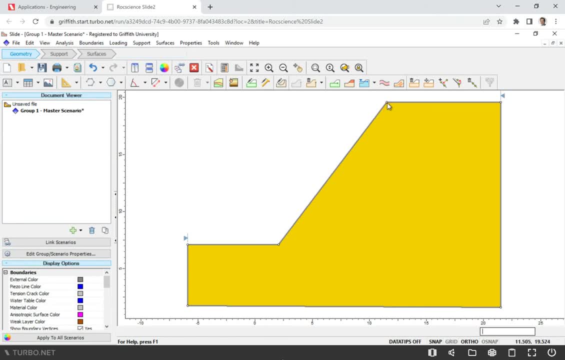 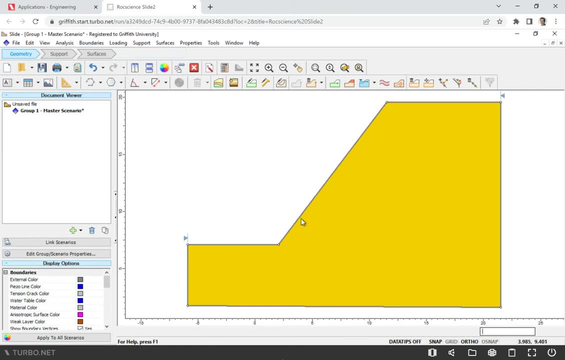 on the right and a bit of space on the left, because when you do slope stability analysis there may be some critical failure planes that will actually go and pass the top. so just always add something to the left and something to the right. okay, so if you are not really satisfied with the slope the way that, 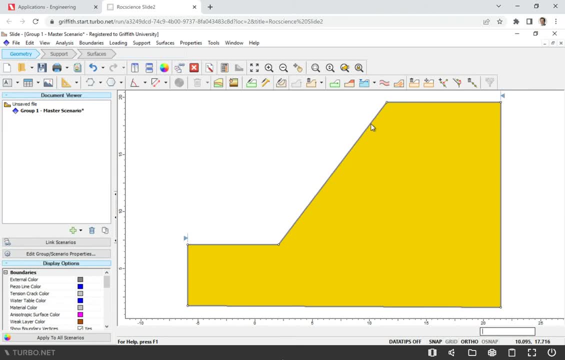 coordinates, so the way to do it. so you right click on the shape and it says here edit coordinates. so you have this table and you can adjust all the coordinates. let's say i don't like the first point, maybe make it negative six, right click, ok, so i think it moved a little bit. another point is: 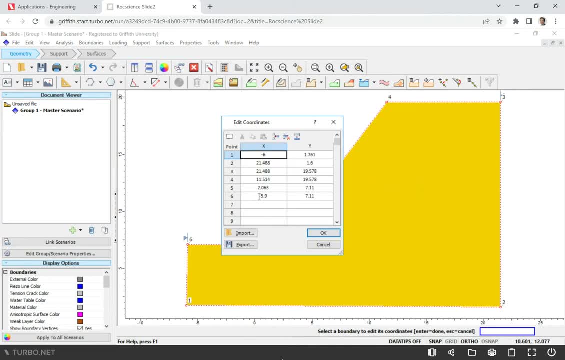 you can add more points. you can add points to make it more accurate your cross section, your profile. um, what i want to do right now just want to change. i want to move this point, make it perpendicular, and now i'm very happy. so i'm very happy with the slope. that's what i wanted. 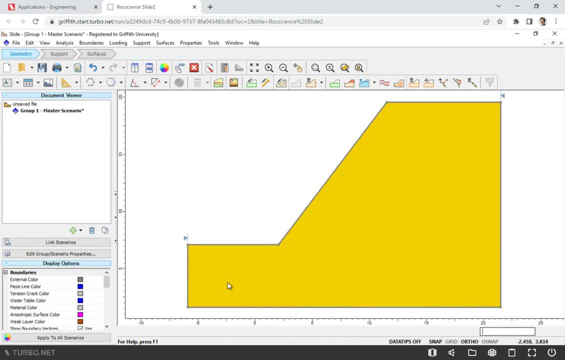 to investigate. okay, so next point is: we're going to draw different layers of rocks um. for this particular case, let's have just, uh, two layers of rocks and i'm gonna go to boundaries and add material boundary, um, and this draw boundary like this: right click, right click mouse, done, okay, so this will be. 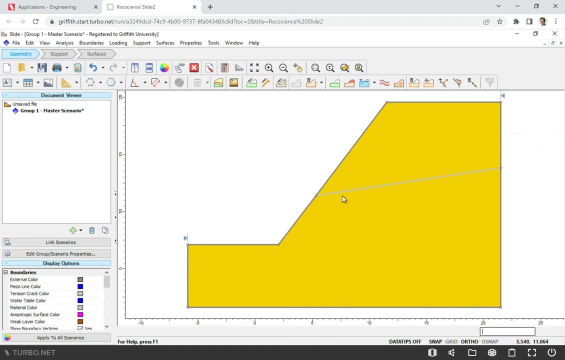 top layer, bottom layer. how do you know where to draw this boundary? well, you should look at your cross section and you should look at your borehole logs. in the borehole logs you will see the depth of each layer. so you have to measure the depth from the surface to make it accurate. 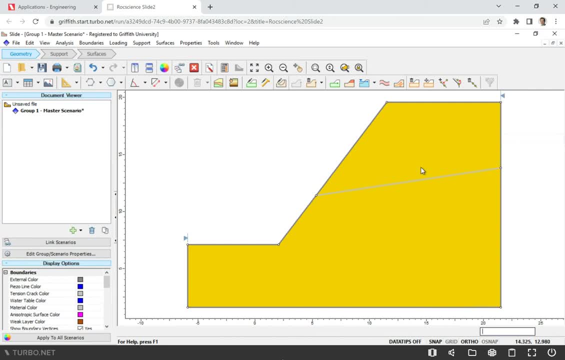 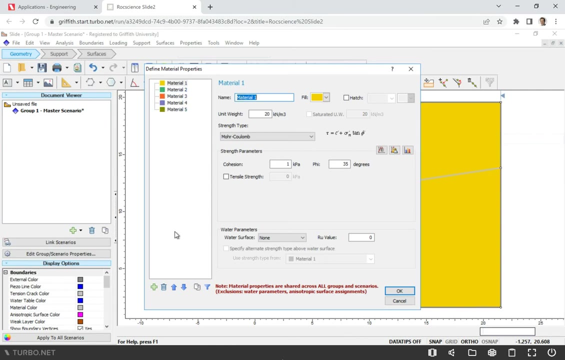 okay, so i drew the boundary. now i'm going to assign properties to these two layers and make them different. i'm going to go to properties and define materials. so i already have five different materials that i can recycle. if, let's say, i have slope with more than five materials, i can always add another one. material six: 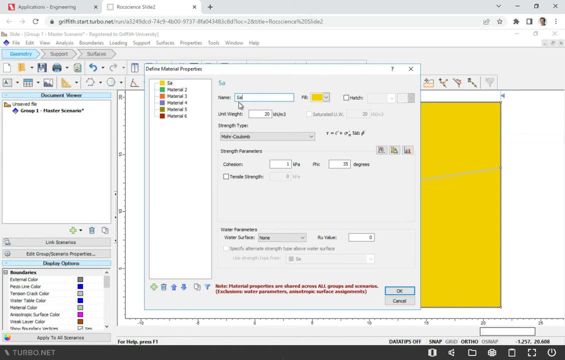 so let's say that material one is sandstone and it has unit weight of, let's say, 23.. we're going to use more cologne failure criteria. so this is the formula. you see, there is different options. sometimes you can even go with cook brown. so i'm you, can i watch my vidéos? 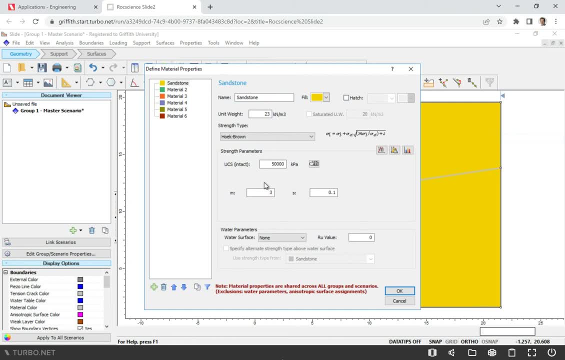 video on rock data: how to use hook brown failure criteria to get cohesion and friction angle. so i believe this option is already built in. you will have to just change mi, which will be the one for sandstone- i believe it's 17- and then you'll need to provide unconfined compressive strength here. 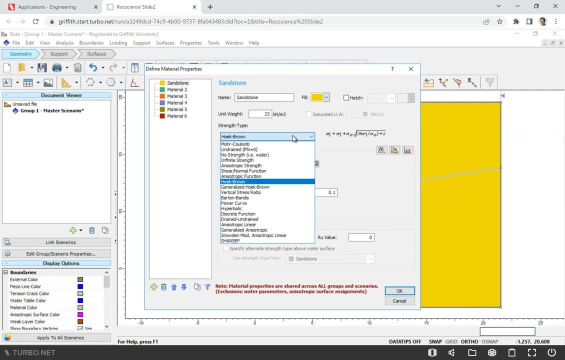 so and then it will estimate cohesion friction angle. i'm gonna do go with just more cologne, and typically we should already have some value of cohesion and friction angle. let's say that it's very weathered sandstone and it has some pretty low cohesion. just, i'll just put maybe 20 right. so 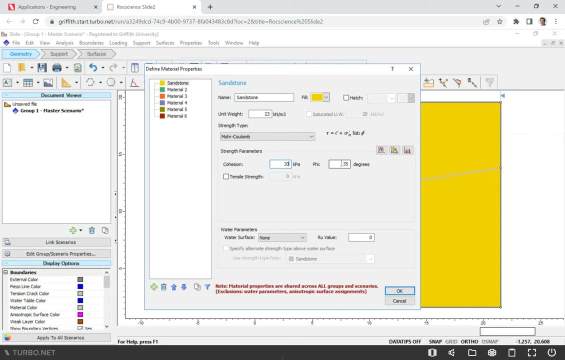 i don't have any data, just i'm like make up these numbers and friction angle is 35 where you can get these numbers. you get these numbers from a laboratory test or from reports. this is something that you really need to know so that you can run this analysis. so i'm going to click ok. 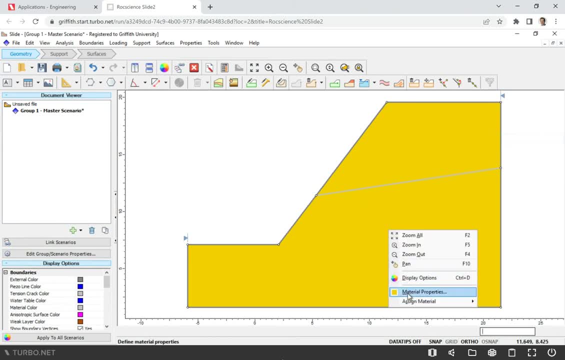 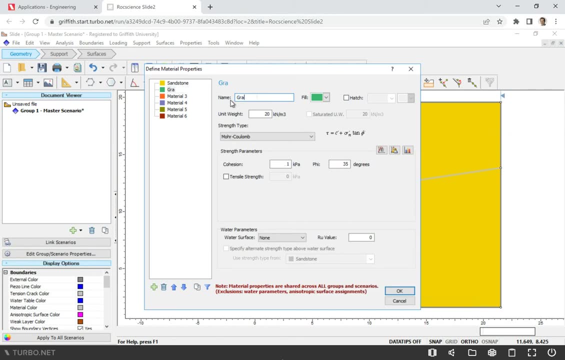 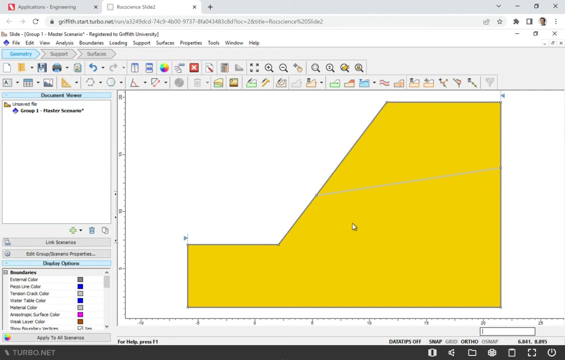 and okay, let's go back material properties. and the second material, let's make it really hard. maybe granite, and that's fresh granites. put maybe 27 um cohesion, because it's really fresh- can be 3 mpa and friction angle 45, it's okay. so now i have two layers. what i'm going to do here, right click at on the bottom. 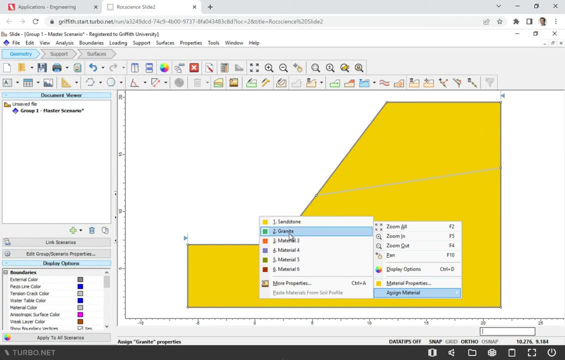 layer and you see this, assign material and i'm going to assign granite. so what i have now? i have sandstone on the top and granite at bottom. so before i do analysis, i'm going to also draw groundwater level right. so let's say that sandstone is very porous. 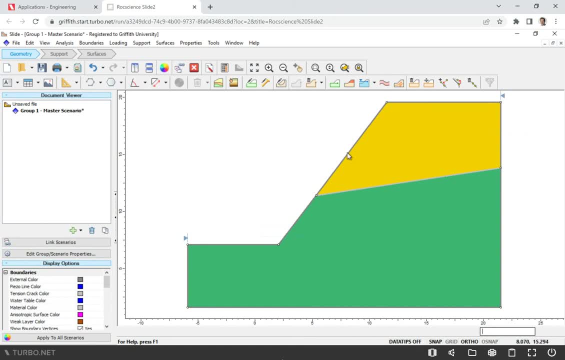 and it's very weathered. so there will be ground water table in sandstone, but not in granite, because granite is very fresh and there is no water there. so what i will do? i'll go to boundaries again, add water table. well, i don't know exactly where ground water day, just draw it somewhere like this: 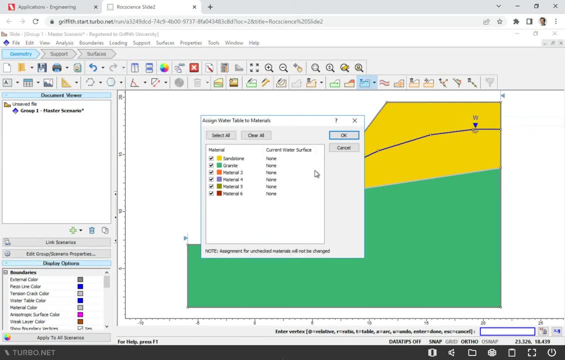 and then right click done and it's ask: so ground water will be in all the materials, and i'm gonna say, no, uh, i'm gonna say that it's only in sandstone. so ground water level only in sandstone, okay. so, uh, now we're ready to do uh. 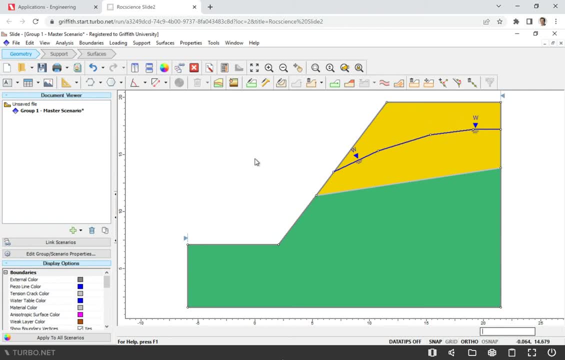 analysis um, the option that i like using for um slope stability analysis. it's called gross surfaces and outer grid. you see, currently it's not available. it's grayed out. so before in the previous slide it was available. but the way to get it back, you just go to surface options. uh, you will select a circular. 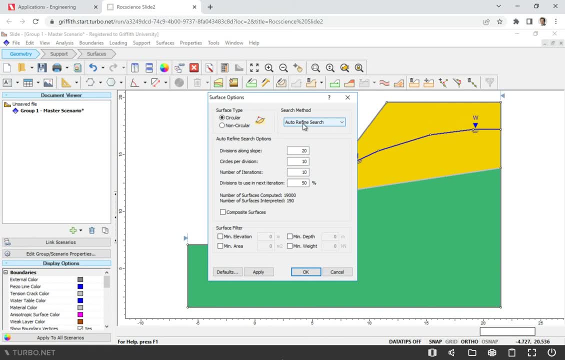 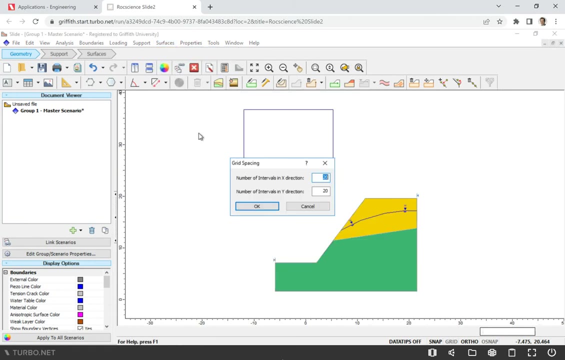 failure plane, so it's already a preset- and then go here and click grid search and click ok. so now when you go here- uh surfaces, you will see that you can use outer grid and that's what i'm going to use. um, you can change the spacing. from my experience, 20 by 20. it's very good, so don't really need to. 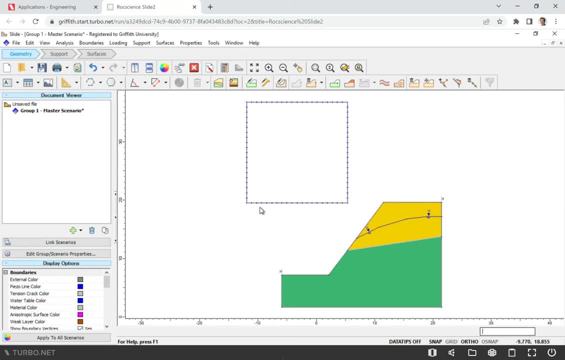 change much, i'm going to click ok, it's not going to make it. um, if you change it, let's say 30 to 30, it's not going to make it any better. it's going to be like same data. and now i'm going to go to. 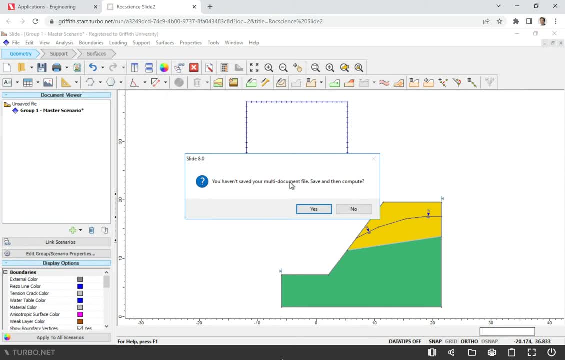 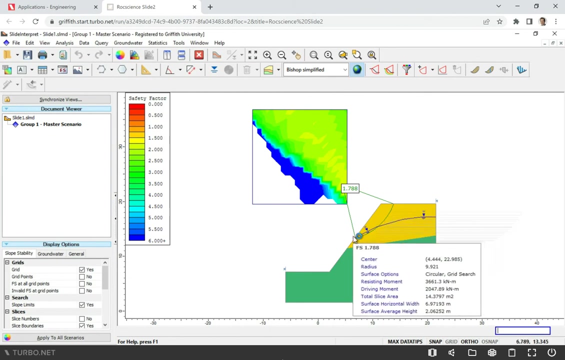 compute. you can go analysis and compute. well, i need to save it, click save and i'm going to do compute. so it's pretty quick. and now i'm going to look at the results, analysis and interpret. so let's see what we have here. okay, so you see that this is the failure plane. software will give you failure plane with the. 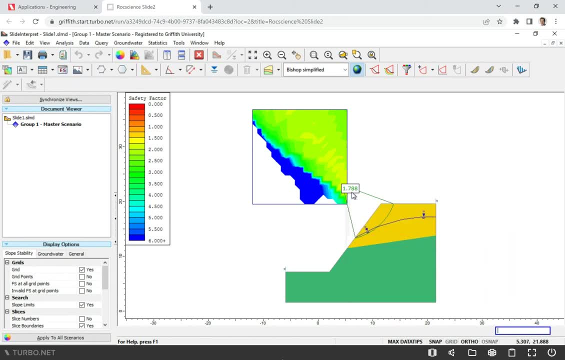 most critical safety factor. it's 1.79, so this is more than one, which means that it's stable. what you can do is you can look at different surfaces. so if you click this one, all surfaces, so this, all the surfaces, that software consider it right and out of all these surfaces it found.